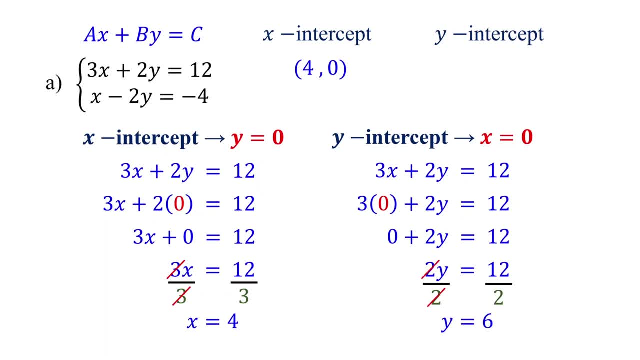 by 2.. Cancel out the 2s. 12 divided by 2 is 6.. the y-intercept occurs when x is 0 comma 6.. This product is called a central makinghosic junt. When x is the vital clue, with your k couldn't I use a. 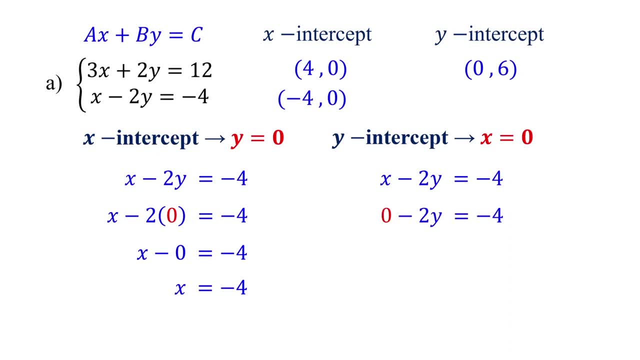 new look. Cancel out the 1s on the x-intercept. Now let's find the intercepts for the second equation. Replace y to 0.. To find the x-intercept, 2 times 0 equals 0, and we get x equals negative 4.. To find the x-intercept. 2 times 0 equals 0, and we get x equals negative 4.. So the x-intercept of the second equation is negative 4 comma 0.. Set x to 0 to find the y-intercept. Divide both sides of the equation with a minus 0 to 4, That will give us a max 2.. 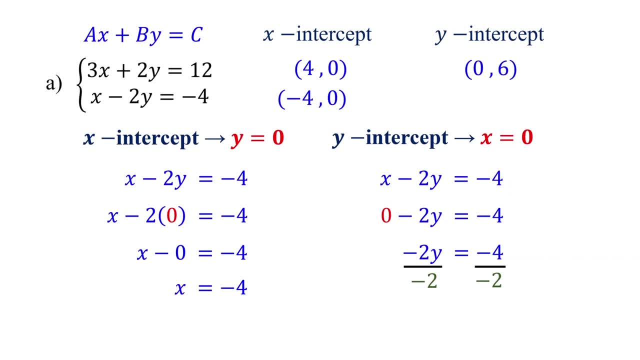 Divide both sides by negative 2 to isolate y. Negative 4 divided by negative 2 is 2, giving us the y-intercept. Now that we have our intercepts for both equations, the next step is to plot them on a graph. 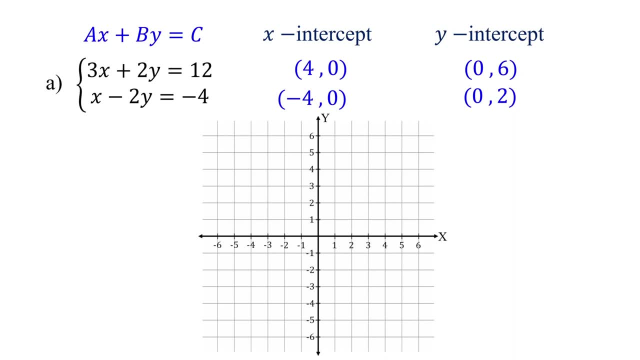 For the first equation plot the x-intercept which is at, and the y-intercept which is at, Then connect the two points with a straight line. This line represents the first equation For the second equation plot, which is the x-intercept and which is the y-intercept. 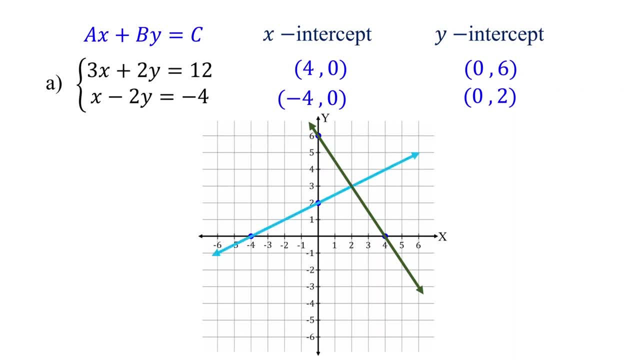 Then connect them with a straight line. This is the line of the second equation, The intersection point of these two lines, which is is the solution to the system of equations. We can verify this solution by substituting it into both equations, Substitute 2 for x and 3 for y. 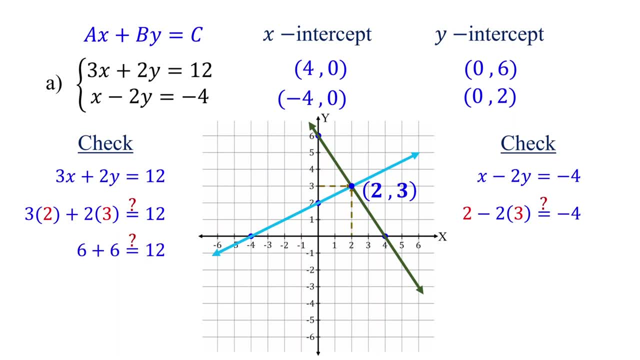 In the first equation, 3 times 2 is 6, and 2 times 3 is also 6,, which adds up to 12.. In the second equation, 2 times 3 equals 6, and 2 minus 6 equals negative 4.. 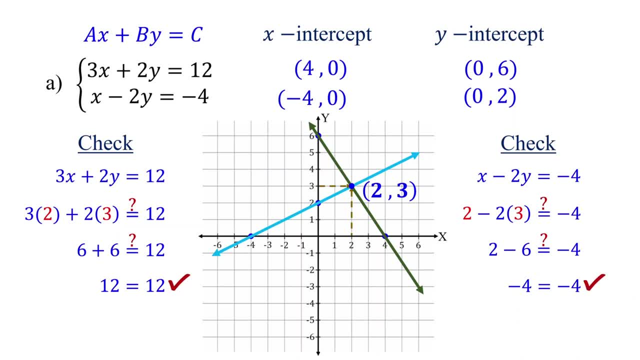 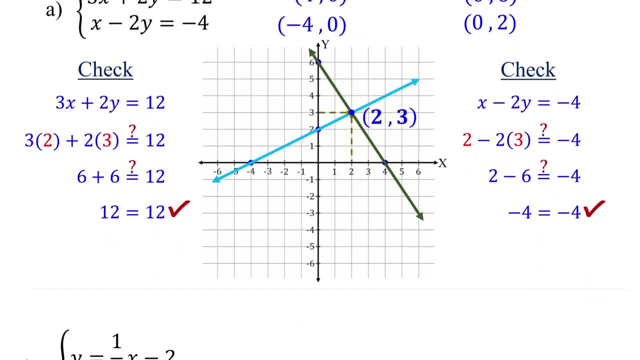 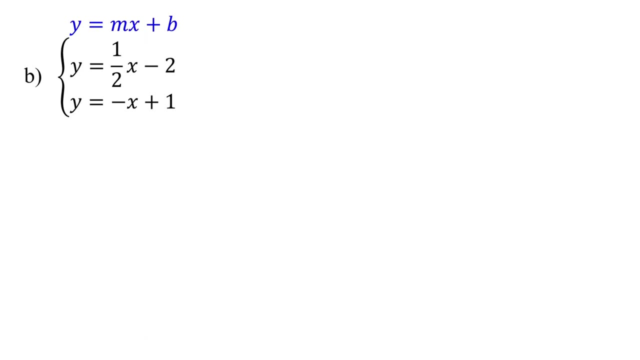 As you can see, both equations are satisfied, confirming that the order pair is indeed the solution. Now let's solve the second example, where the equations are given in slope-intercept form. To graph an equation in slope-intercept form, the most straightforward method is to use the y-intercept and the slope. 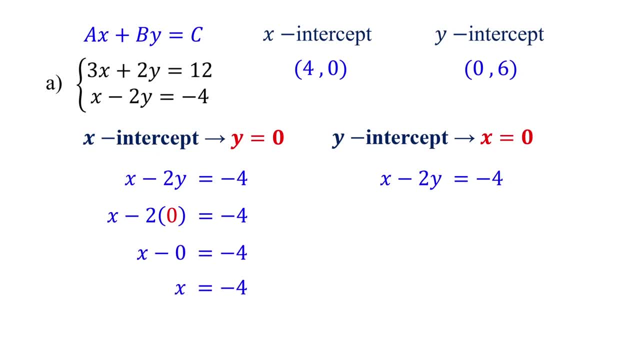 2 times 0 equals 0, and we get x equals negative 4.. So the x-intercept of the second equation is negative, 4 comma zero. Set x to zero to find the y-intercept. Divide both sides by negative 2 to isolate y. 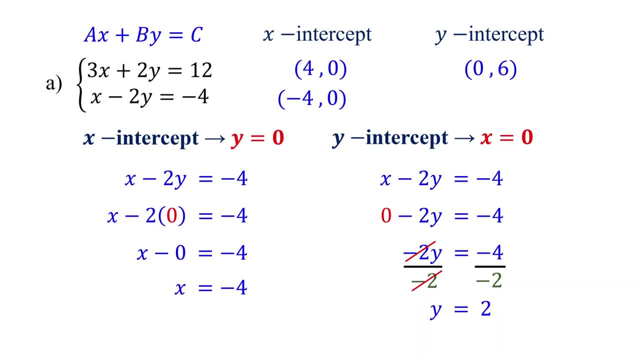 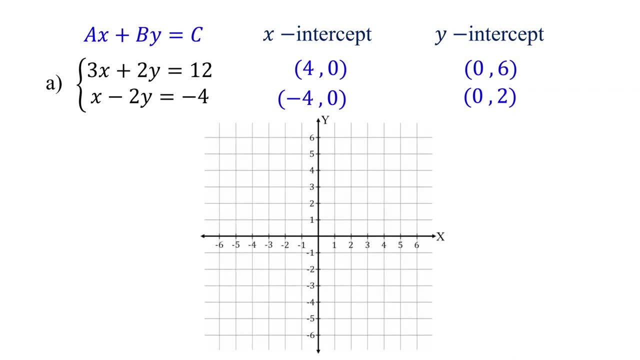 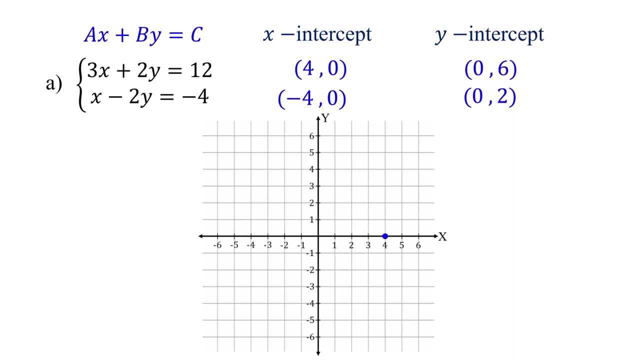 Negative 4 divided by negative 2 is 2, giving us the y-intercept. Now that we have our intercepts for both equations, the next step is to plot them on a graph. For the first equation, plot the x-intercept which is at and the y-intercept which is at. 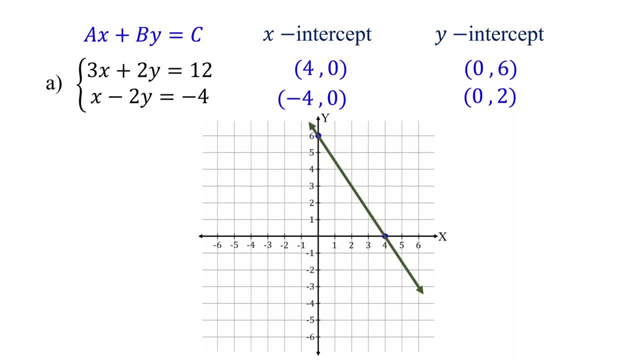 Then connect the two points with a straight line. This line represents the first equation. For the second equation, plot which is the x-intercept and which is the y-intercept. Then connect them with a straight line. This is the line of the second equation. 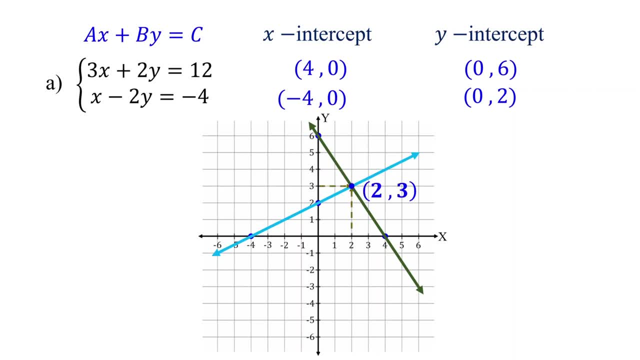 The intersection point of these two lines, which is is the solution to the system of equations. We can verify this solution by substituting it into both equations. Subtract the x-intercept and the y-intercept, Substitute 2 for x and 3 for y. 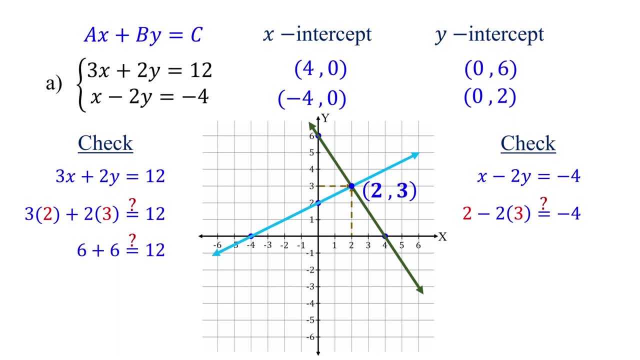 In the first equation, 3 times 2 is 6, and 2 times 3 is also 6,, which adds up to 12.. In the second equation, 2 times 3 equals 6, and 2 minus 6 equals negative 4.. 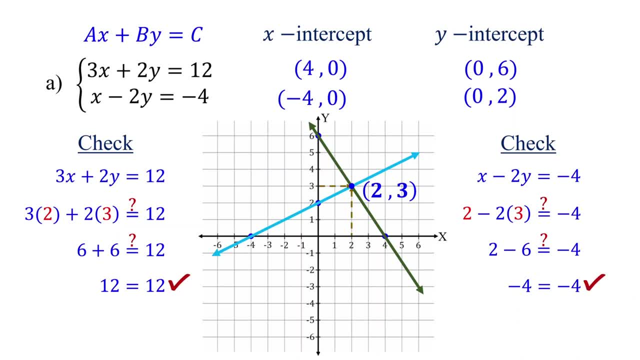 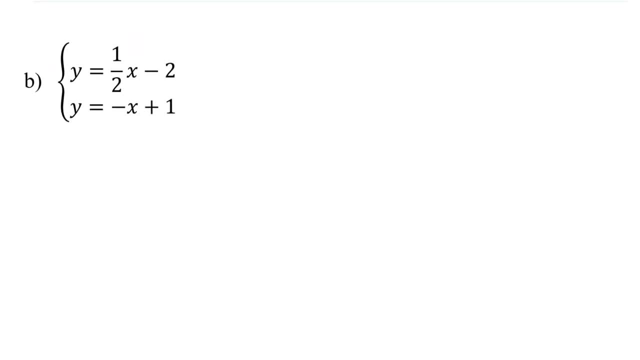 As you can see, both equations are satisfied, confirming that the order pair is indeed the solution. Now let's solve the second example. The equations are given in slope-intercept form. To graph an equation in slope-intercept form, the most straightforward method is to use the y-intercept and the slope. 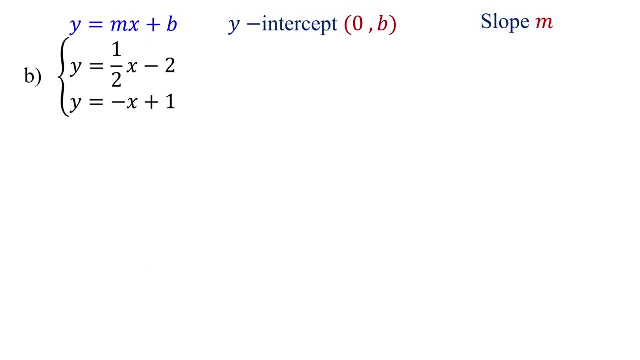 So the first step is to identify these values from the equations. For the first equation, the y-intercept is at and the slope is 1 over 2.. For the second equation, the y-intercept is at and the slope is negative 1.. 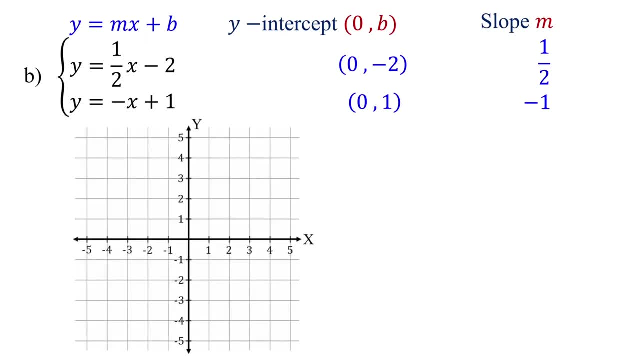 Now let's begin by graphing the first equation. First plot the y-intercept which is located at. Remember that slope is the ratio of rise over ran, Since the slope is 1 over 2, the rise is 1 unit up and the ran is 2 units to the right. 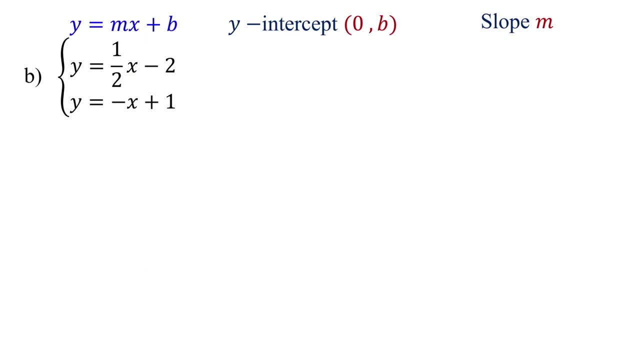 So the first step is to identify these values from the equations. For the first equation, the y-intercept is at and the slope is 1 over 2.. For the second equation, the y-intercept is at and the slope is negative 1.. 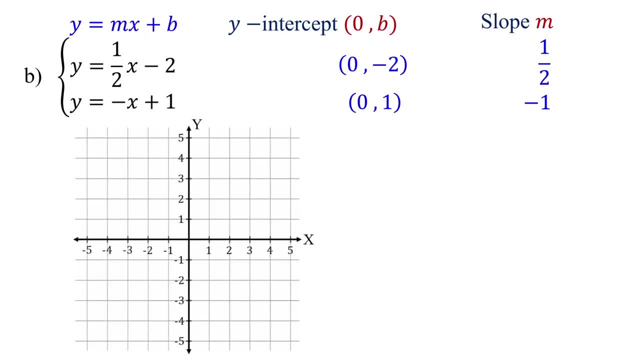 Now let's begin by graphing the first equation. First plot the y-intercept which is located at. Remember that slope is the ratio of rise over ran, Since the slope is 1 over 2, the rise is 1 unit up and the ran is 2 units to the right. 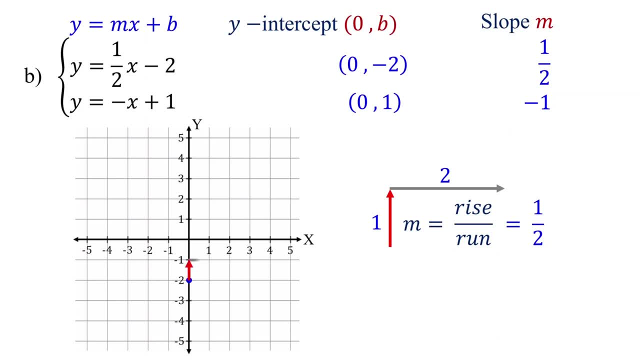 Now, starting from the y-intercept, go up 1 unit, then move to the right 2 units. Plot this as the second point. Let's plot one more point, Starting from this point: again go up 1 unit and to the right 2 units. 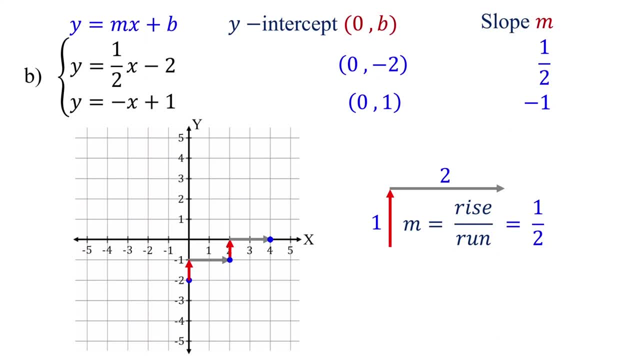 Then plot this as the third point. The advantage of the slope-intercept form is that we can easily plot more points and make our graph more accurate. Next, connect the points with a straight line. This represents the line of the first equation. 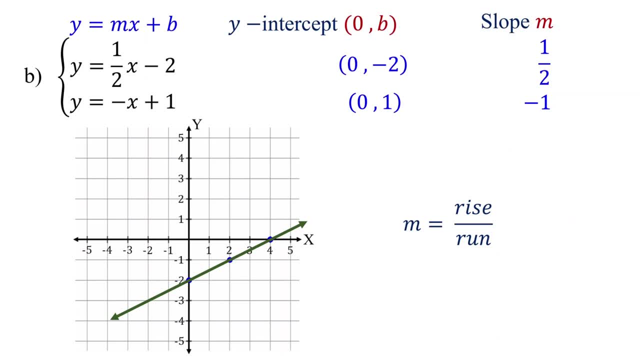 Now let's plot the graph of the second equation, As we did before. we start by plotting the y-intercept, which is located at Its slope, is negative 1,, which is the same as negative 1 over 1, right. 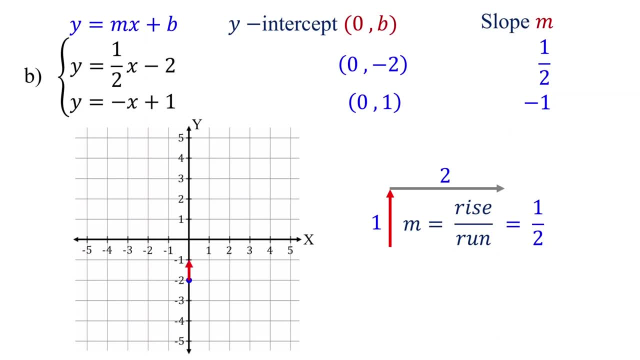 Now, starting from the y-intercept, go up 1 unit, then move to the right 2 units. Plot this as the second point. Let's plot one more point, Starting from this point: again go up 1 unit and to the right 2 units. 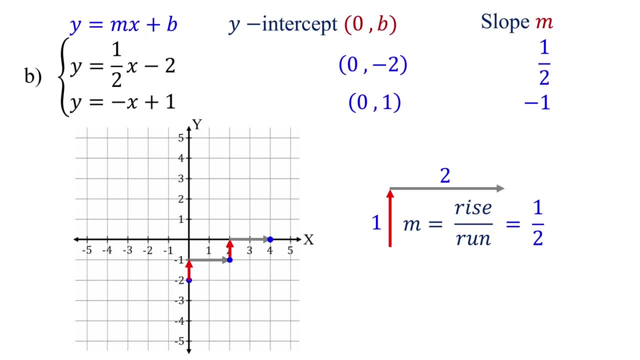 Then plot this as the third point. The advantage of the slope-intercept form is that we can easily plot more points and make our graph more accurate. Next, connect the points with a straight line. This represents the line of the first equation. 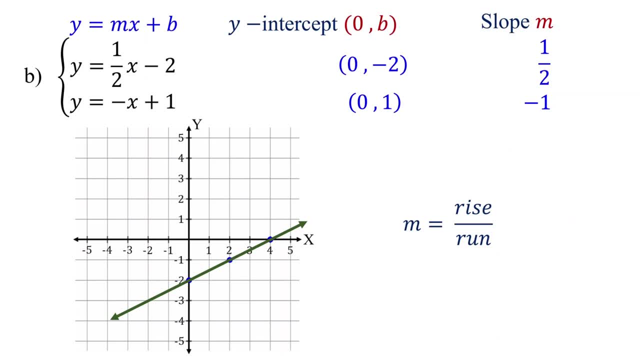 Now let's plot the graph of the second equation, As we did before. we start by plotting the y-intercept, which is located at Its slope, is, which is the same as right. So the rise is 1 unit down and the run is 1 unit to the right. 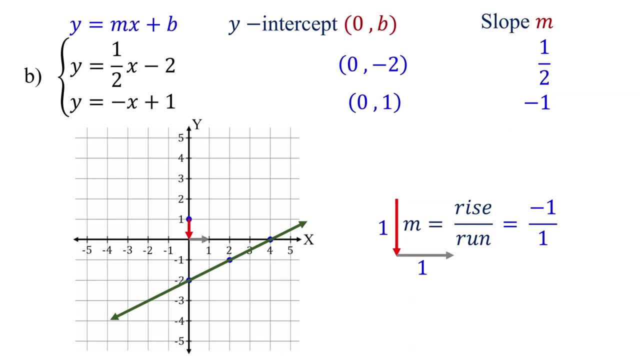 Starting from the y-intercept, go down 1 unit, then move to the right 1 unit. Plot one more point by moving from this point: 1 unit down and 1 unit right Now. connect these points with a straight line. 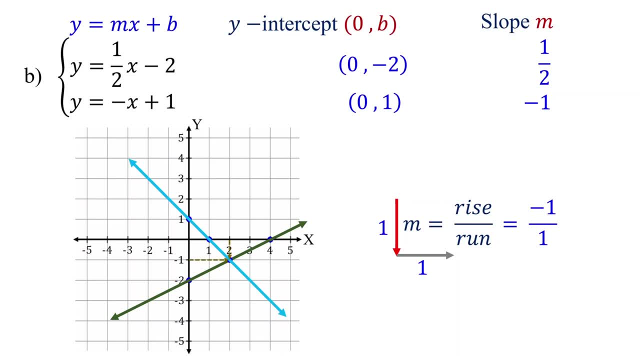 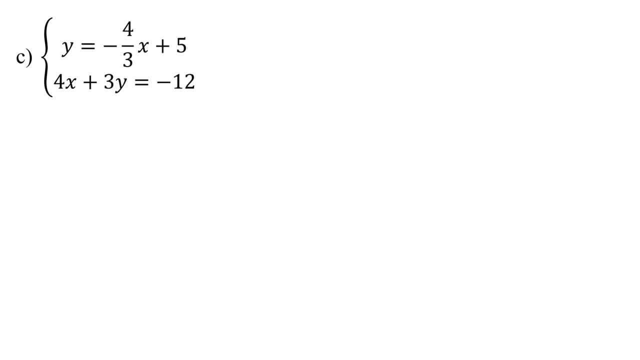 This is the line of the second equation. The intersection point of the two lines is: which is the solution to the system of equations? If you have any questions, please feel free to leave them in the comments below. Now let's consider the two special cases. 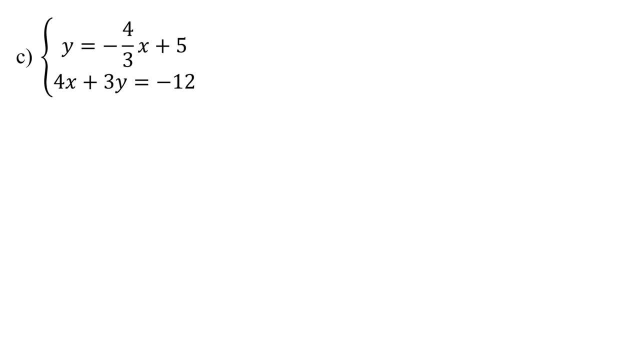 What method do you suggest to graph these equations? The first equation is given in slope-intercept form, so you can use the y-intercept and the slope, while the second equation is given in standard form, so you can use the intercept method. 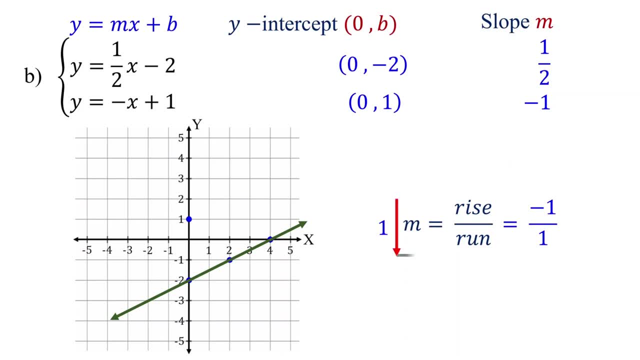 So the rise is 1 unit down and the run is 1 unit to the right. Starting from the y-intercept, go down 1 unit, then move to the right 1 unit. Plot one more point by moving from this point: 1 unit down and 1 unit right. 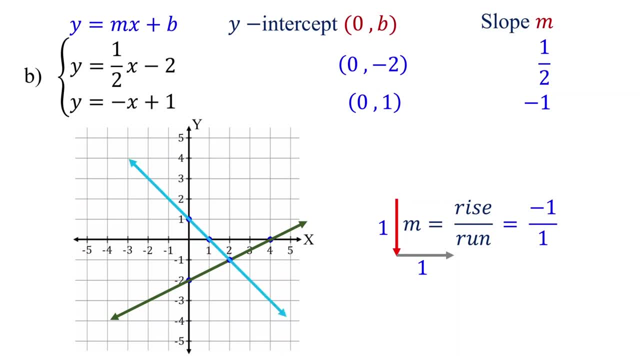 Now connect these points with a straight line. This is the line of the second equation. The intersection point of the two lines is, which is the solution to the system of equations. If you have any questions, please feel free to leave them in the comments below. 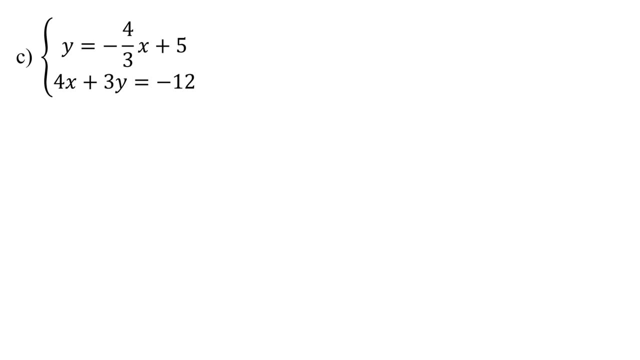 Now let's consider the two special cases. What method do you suggest to graph these equations? The first equation is given in slope-intercept form, so you can use the y-intercept and the slope, while the second equation is given in standard form. 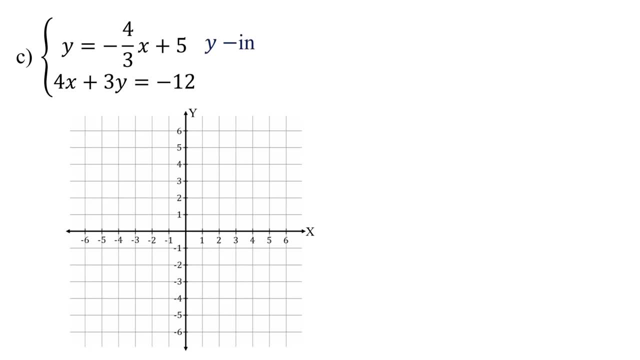 so you can use the intercept method. The y-intercept of the first equation is the point and the slope is negative, 4 over 3.. As we did in the previous example, we will start by plotting the y-intercept, which is located at. 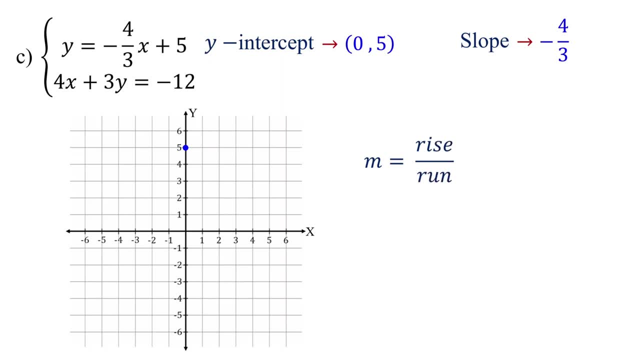 Slope is rise over run and in this case it is negative: 4 over 3.. You can place the negative sign in the numerator. It will not change the value of the slope, since they are equivalent fractions. The key concept to remember is that: 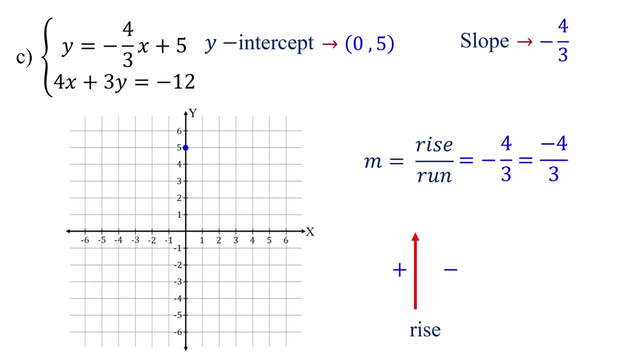 when the rise is positive, we move up, and when it is negative, we move down. In this case, since the rise is negative, 4,, we move 4 units down. Similarly, when the run is positive, we go to the right. 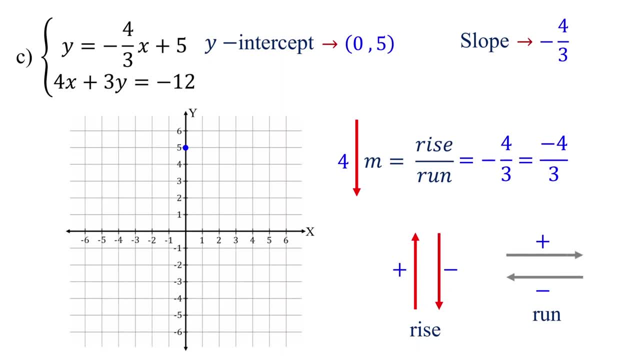 and when it is negative we go to the left. In this case, the run is positive 3, so we go 3 units to the right. Now, starting from the y-intercept, move down 4 units, then move to the right 3 units. 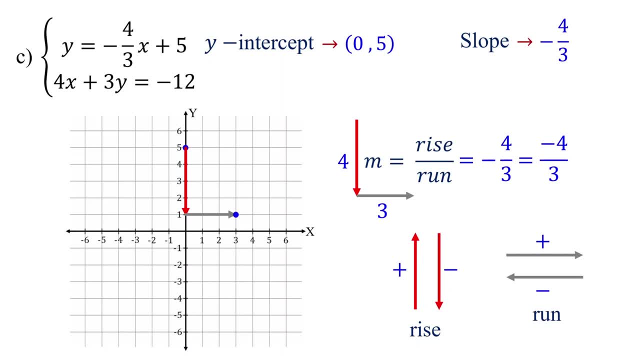 and plot the second point. Let's add one more point. Starting from this point, move down 4 units and move to the right 3 units and plot the third point. Then connect these points with a straight line. Now let's move on to graphing the second equation. 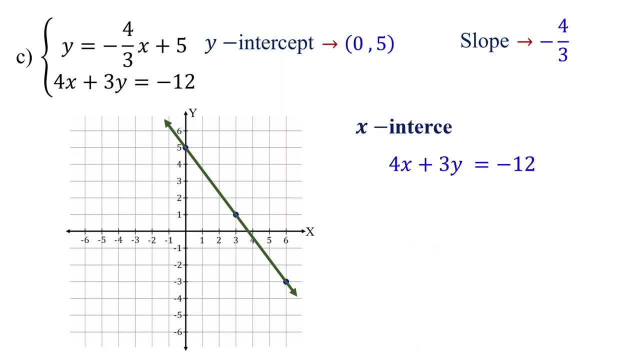 using the intercept method. First let's find the x-intercept. Set y to 0 and solve for x: 3 times 0 equals 0, so we are left with 4x equals negative 12.. Dividing both sides of the equation by 4,: 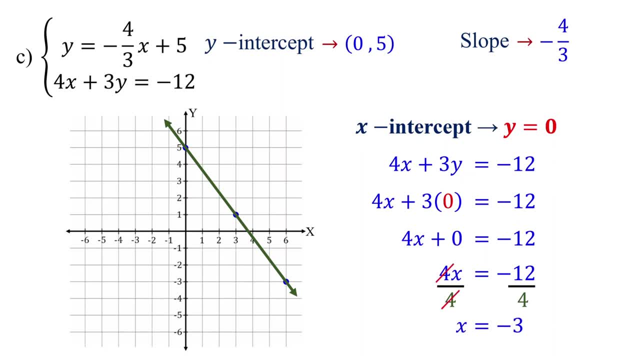 we get: x equals negative 3. So the x-intercept is negative, 3 comma 0.. Next let's find the y-intercept by setting x to 0 and solving for y 4 times 0 equals 0,. 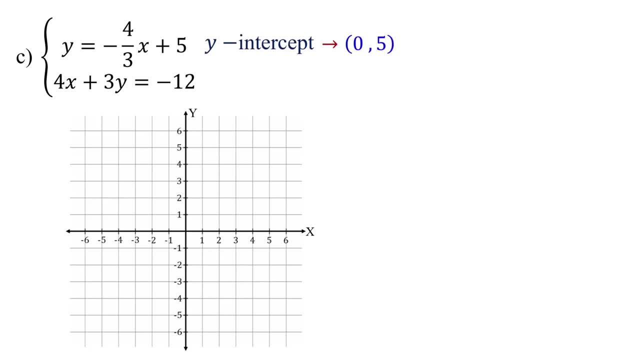 The y-intercept of the first equation is the point and the slope is. As we did in the previous example, we will start by plotting: the y-intercept, which is located at Slope is rise over run and in this case it is. 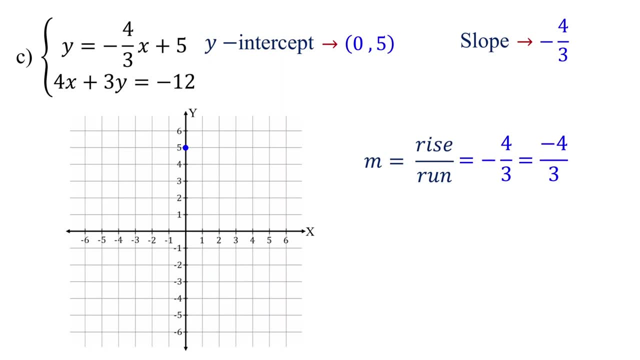 You can place the negative sign in the numerator. It will not change the value of the slope, since they are equivalent fractions. The key concept to remember is that when the slope of the first equation is 0, we move up, and when it is negative, we move down. 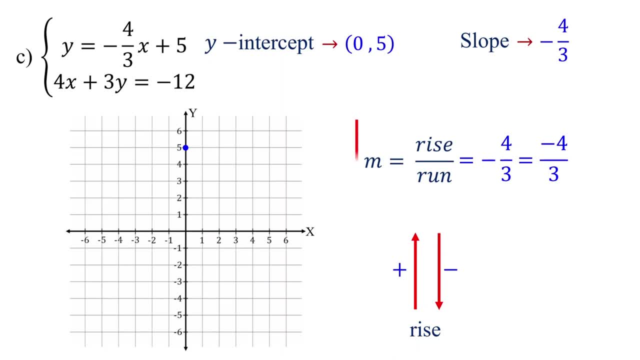 In this case, since the rise is, we move 4 units down. Similarly, when the run is positive, we go to the right and when it is negative we go to the left. In this case, the run is positive 3, so we go 3 units to the right. 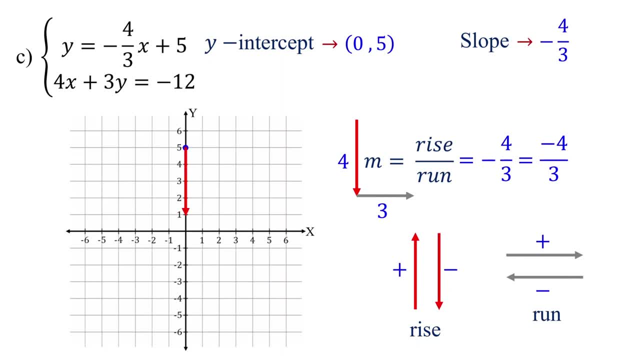 Now, starting from the y-intercept, move down 4 units, then move to the right 3 units and plot the second point. Let's add one more point. Starting from this point, move down 4 units and move to the right 3 units. 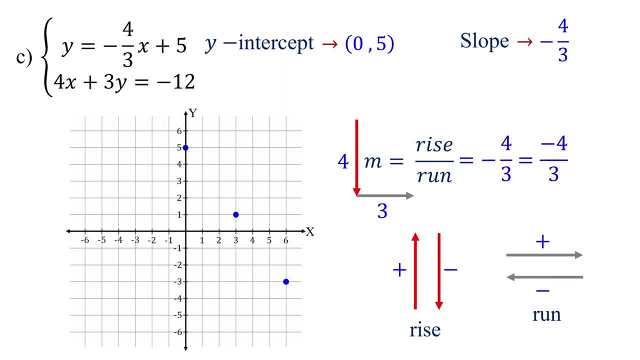 and plot the third point, Then connect these points with a straight line. Now let's move on to graphing the second equation using the intercept method. First let's find the x-intercept, Set y to 0 and solve for x. 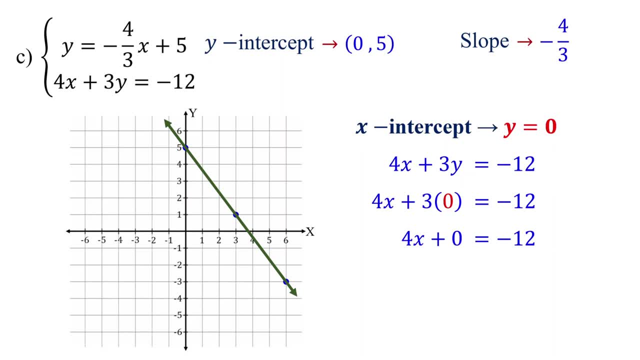 3 times 0 equals 0, so we are left with x equals negative 12. Dividing both sides of the equation by 4, we get x equals negative 3. So the x-intercept is negative. 3 comma 0. 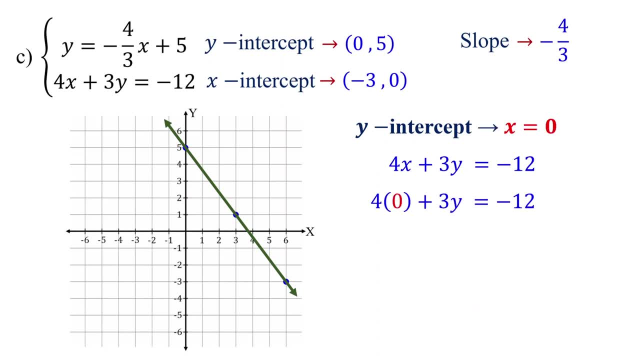 Next let's find the y-intercept by setting x to 0 and solving for y 4 times 0 equals 0, and we get 3y equals negative 12.. To isolate y, divide both sides by 3,. 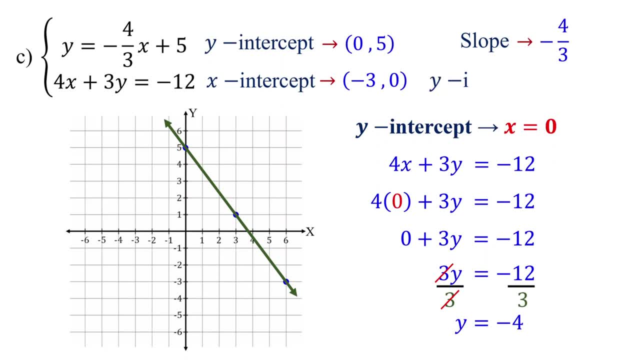 giving us y equals negative 4.. Therefore, the y-intercept is 0 comma negative 4.. Now plot the x-intercept, which is located at negative 3 comma 0,, and the y-intercept, which is at 0 comma negative 4.. 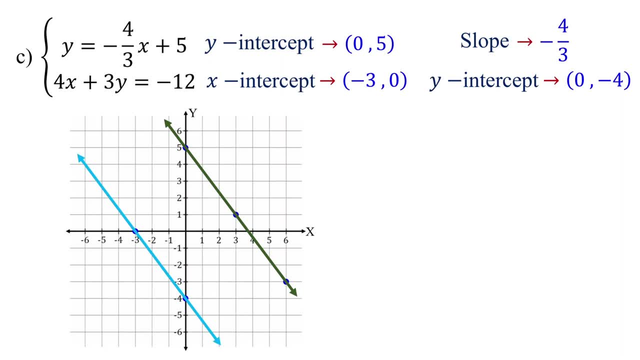 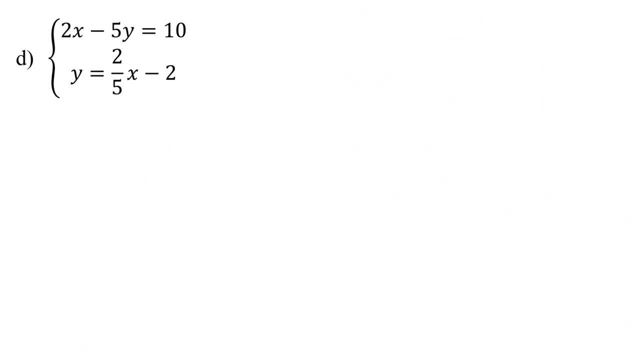 Then connect these two points with a straight line. Notice that the two lines do not intersect. they are parallel lines. If the lines of the two equations are parallel, then the system has no solution. Finally, let's consider the case Where the system of equations has infinitely many solutions. 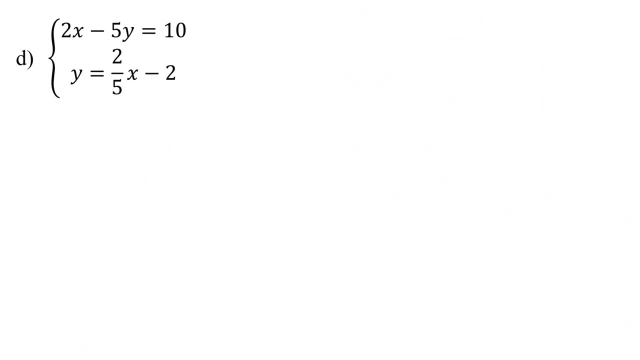 Please feel free to pause the video and give it a try. The first equation is given in standard form, so first we will find its x and y-intercepts. To find the x-intercept, set y to 0.. 5 times 0 equals 0,. 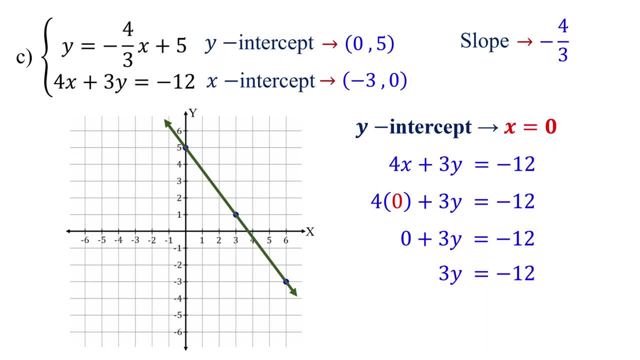 and we get 3y equals negative 12. To isolate y, divide both sides by 3,, giving us y equals negative 4. Therefore the y-intercept is 0 comma negative 4.. Now plot the x-intercept. 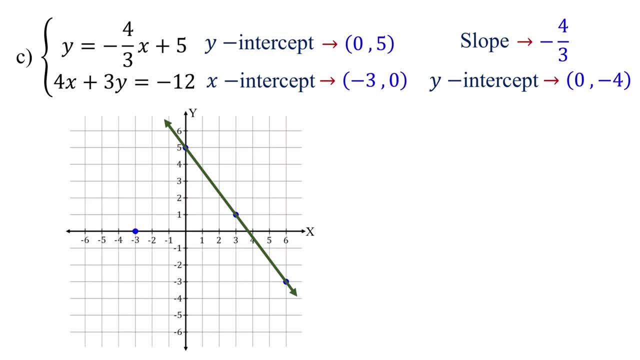 which is located at negative 3 comma 0, and the y-intercept, which is at 0 comma negative 4.. Then connect these two points with a straight line. Notice that the two lines do not intersect, they are parallel lines. 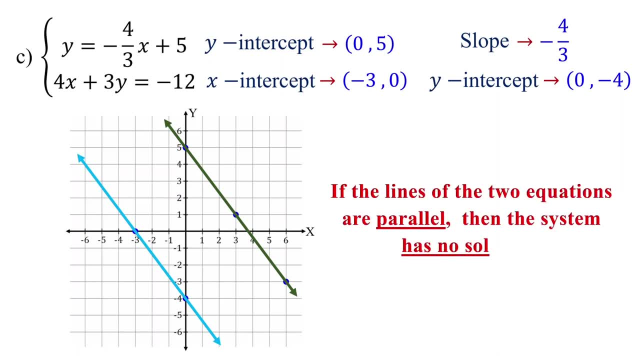 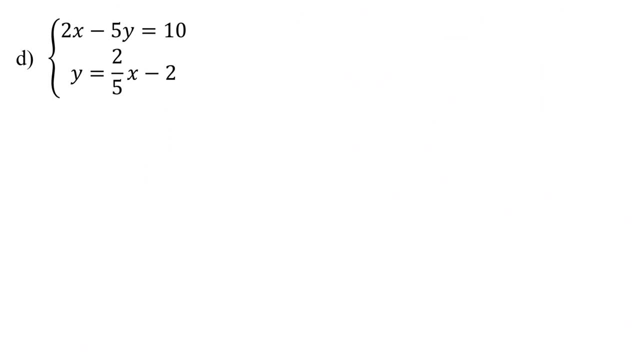 If the lines of the two equations are parallel, then the system has no solution. Finally, let's consider the case where the system of equations has infinitely many solutions. Please feel free to pause the video and give it a try. The first equation is given in standard form. 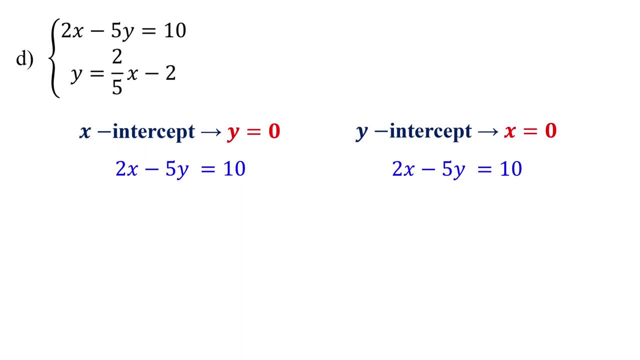 so first we will find its x and y-intercepts. To find the x-intercept, set y to 0.. 5 times 0 equals 0, and we get 2x equals 10.. Divide both sides by 2 to isolate x. 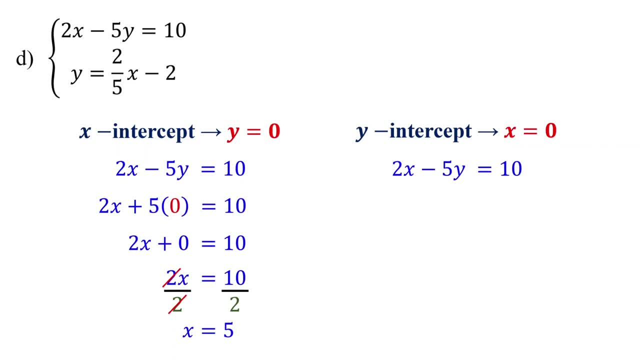 10 divided by 2 is 5.. So the x-intercept is 5 comma 0.. To find the y-intercept, set x to 0.. 2 times 0 equals 0, and we have negative. 5y equals 10.. 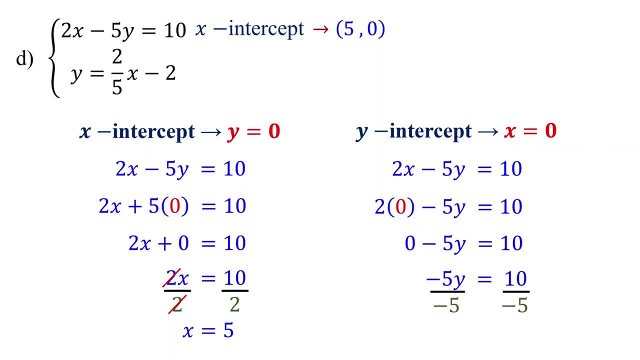 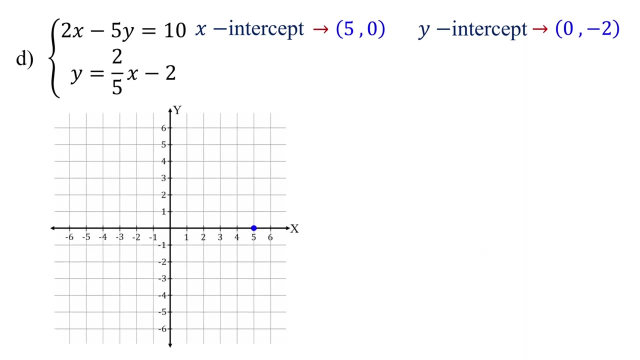 To isolate y, divide both sides by negative 5,, giving us y equals negative 2.. Therefore, the y-intercept is 0 comma negative 2.. Next plot the points on the graph. Plot 5 comma 0, which is the x-intercept. 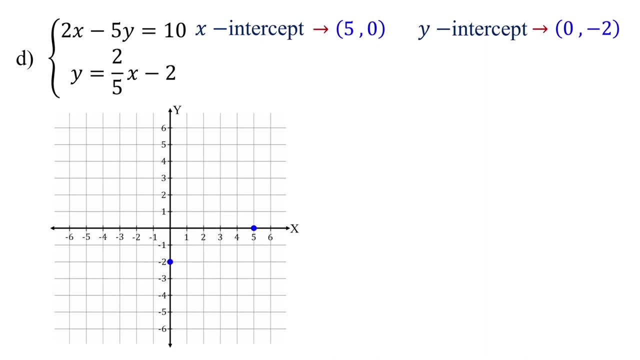 Plot 0 comma negative 2, which is the y-intercept, and then connect them with a straight line. Moving on to the second equation, which is in slope-intercept form, The y-intercept is at 0 comma negative 2,. 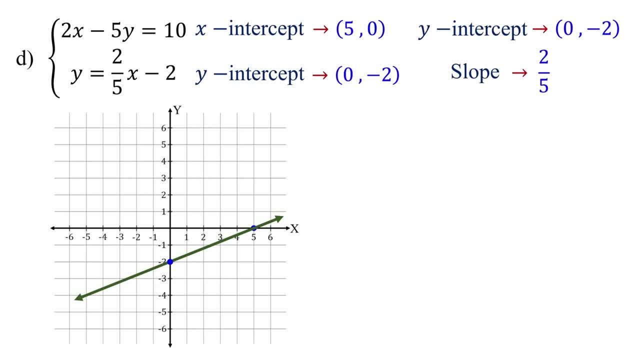 and the slope is 2 over 5.. Start by plotting: the y-intercept Slope is rise over ran and in this case it is 2 over 5, which means the rise is 2 units up and the ran is 5 units to the right. 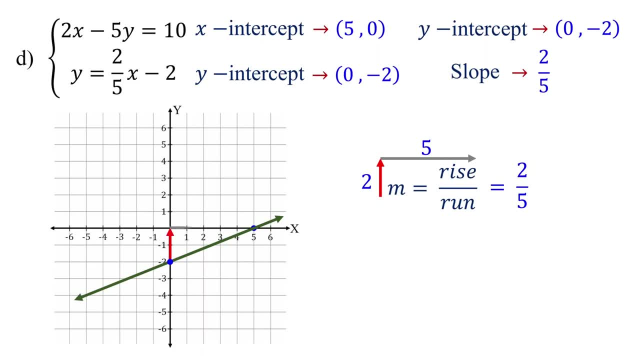 Starting from the y-intercept, move up 2 units, then go to the right 5 units and plot the second point. You have likely noticed that both points lie on the line of the first equation When you connect these points with a straight line. 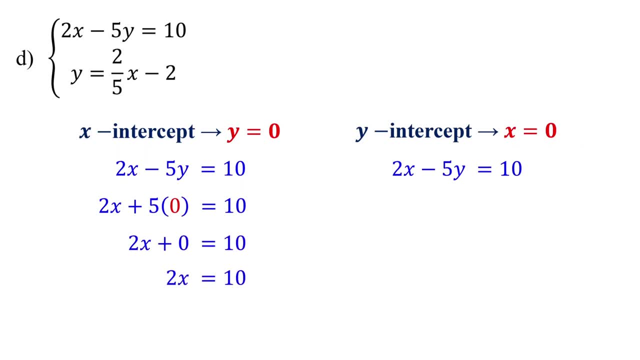 and we get 2x equals 10.. Divide both sides by 2 to isolate x. 10 divided by 2 is 5.. So the x-intercept is 5 comma 0.. To find the y-intercept, set x to 0.. 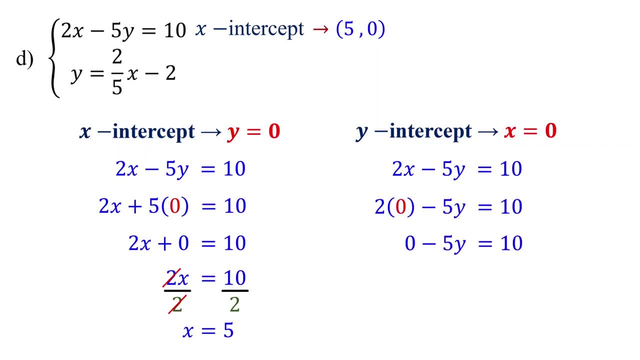 2 times 0 equals 0, and we have negative 5y equals 10.. To isolate y, divide both sides by negative 5,, giving us y equals negative 2. Therefore the y-intercept is 0 comma, negative 2.. 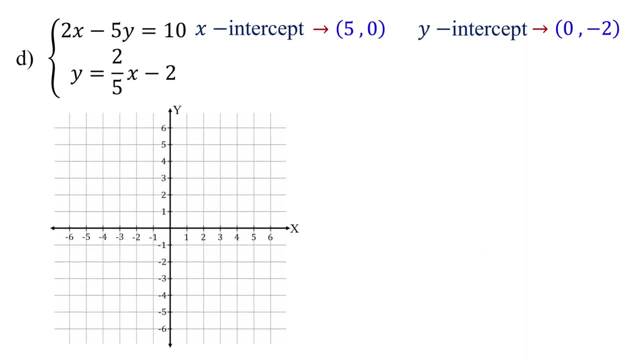 Next, plot the points on the graph: Plot 5 comma 0,, which is the x-intercept, Plot 0 comma negative 2,, which is the y-intercept, and then connect them with a straight line Moving on to the second equation. 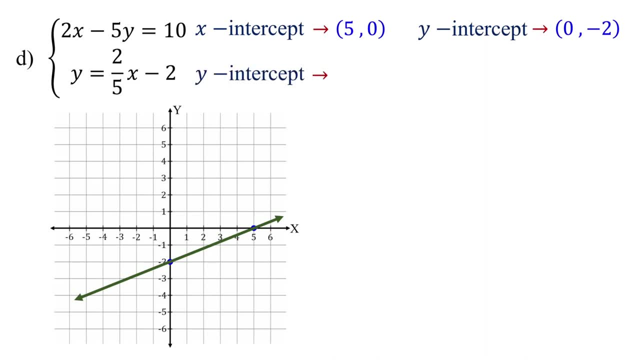 which is in slope-intercept form. The y-intercept is at 0 comma negative 2, and the slope is 2 over 5.. Start by plotting the y-intercept Slope is rise over ran and in this case, 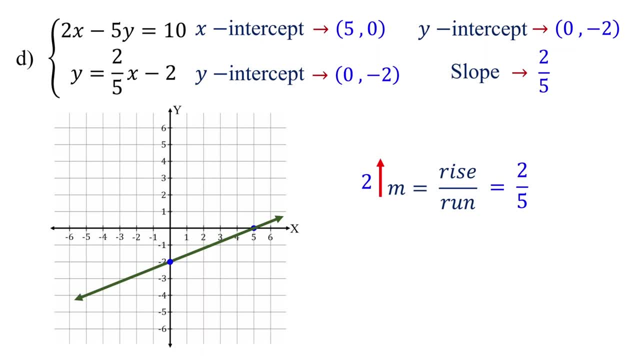 it is 2 over 5, which means the rise is 2 units up and the ran is 5 units to the right. Starting from the y-intercept, move up 2 units, then go to the right 5 units. 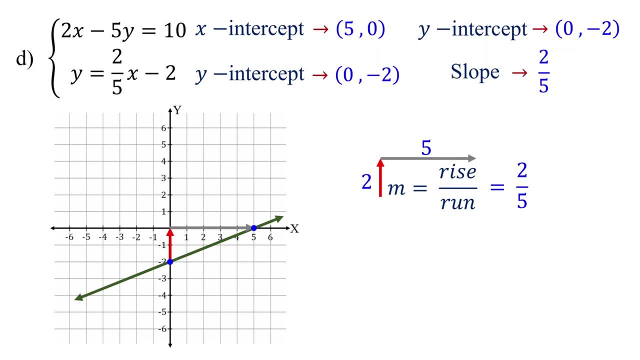 and plot the second point, You have likely noticed that both points lie on the line of the first equation. When you connect these points with a straight line, it perfectly aligns with the first line. So the line of the first equation and the line of the second equation are the same. 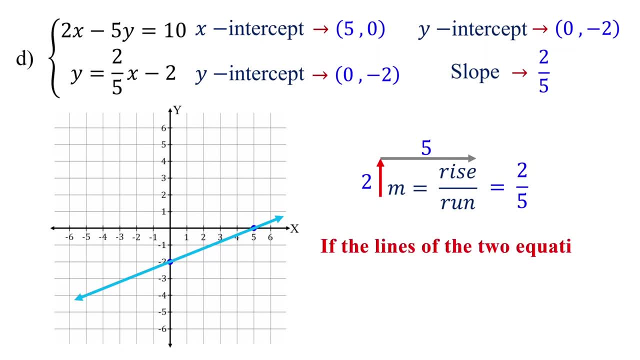 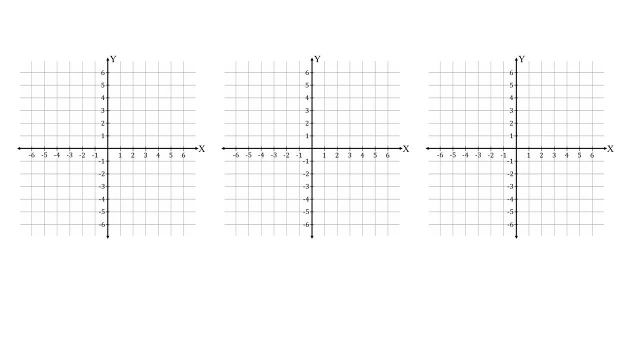 They coincide perfectly. If the lines of the two equations are coincident, then the system has infinitely many solutions. This means that any point on the lines satisfies both equations. In conclusion, when solving a system of equations graphically, first graph each equation on the same coordinate plane. 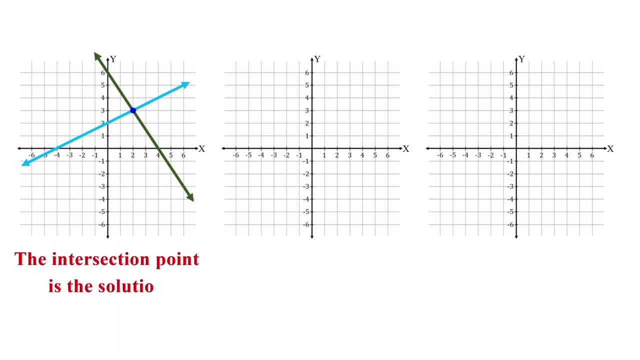 If the lines intersect, the point of intersection is a solution to the system of equations. If they are parallel, the system has no solution. If they are coincident, the system has infinitely many solutions. Thanks for watching. If you found this video helpful. please give it a thumbs up and subscribe.